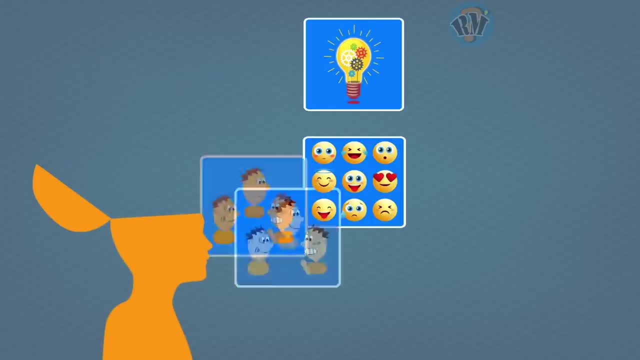 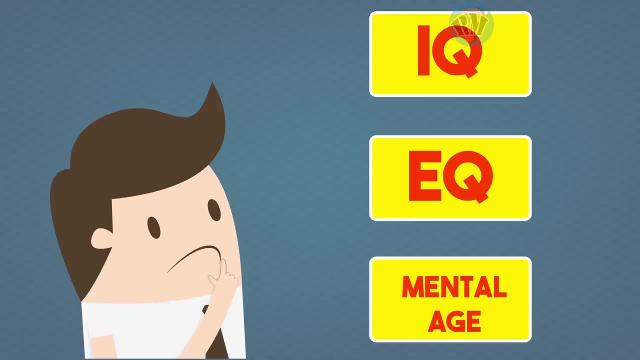 Do you know, our intelligence, emotions and behavior depends on our IQ, EQ and mental age. Do you know your IQ, EQ and mental age? If not, then you are at the right place. We have made a series of three videos in which we will be providing you with all the tests. 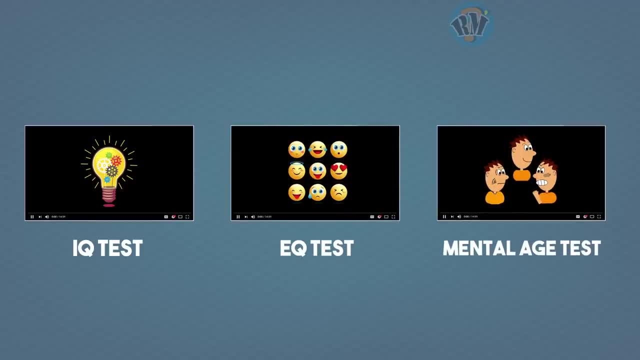 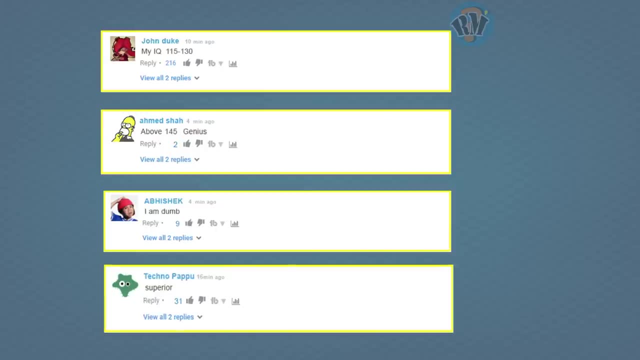 respectively. You can check your IQ level, EQ level and your mental age by giving this test for free, And after completing these tests, please put your scores in the comment box below. To watch more such interesting videos, please subscribe to our channel Griddle Master. 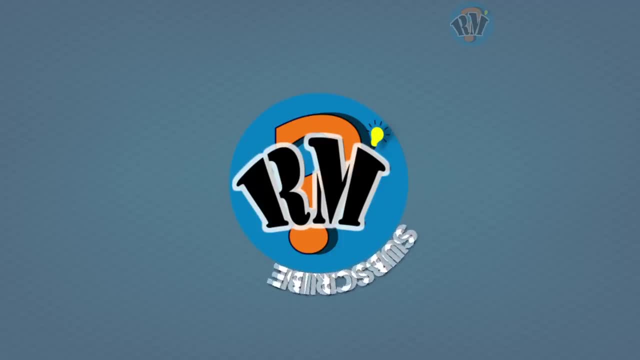 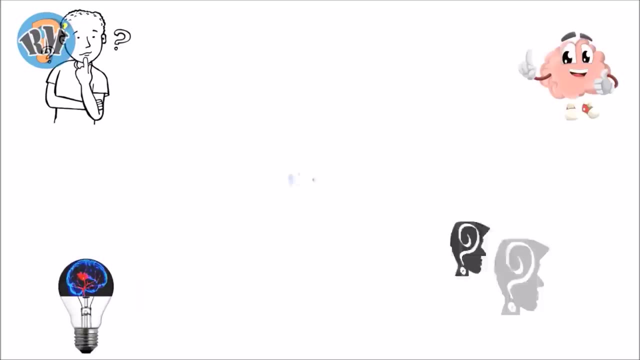 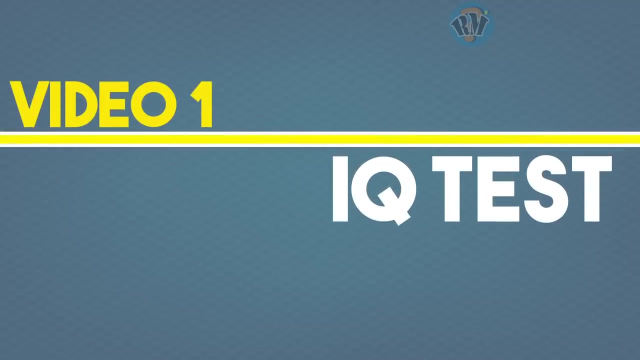 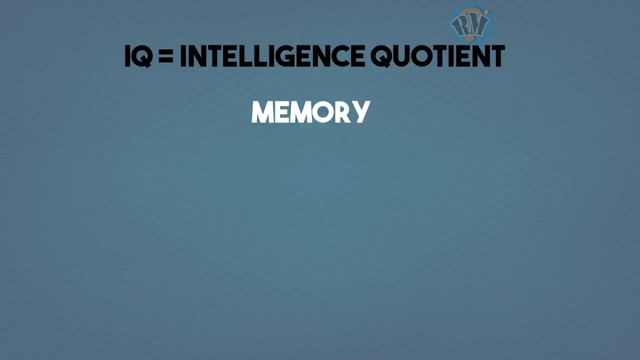 So what are you waiting for? Let's begin the series, Video 1.. In this video, we present you IQ test, And for those who don't know about IQ, here's some fact. IQ stands for Intelligence Quotient. It only defines your memory and 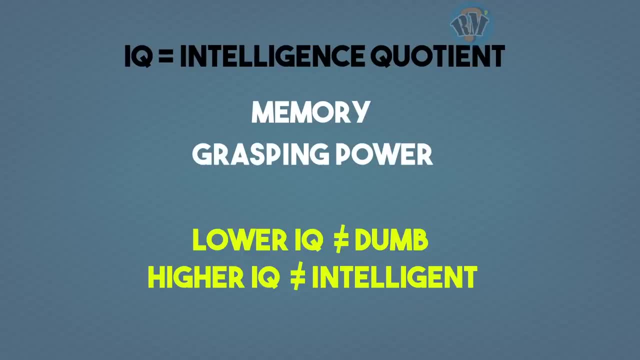 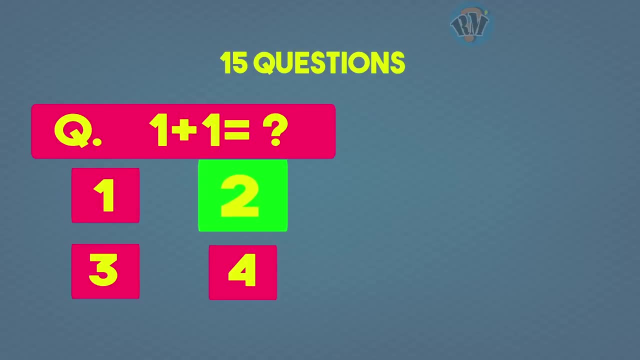 grasping power. Lower IQ does not mean you are dumb. Higher IQ also does not mean you are very intelligent. This test has 15 different types of questions and you have to choose your answers from the provided options. You have 10 seconds to solve each. You will get 1 point for each correct. 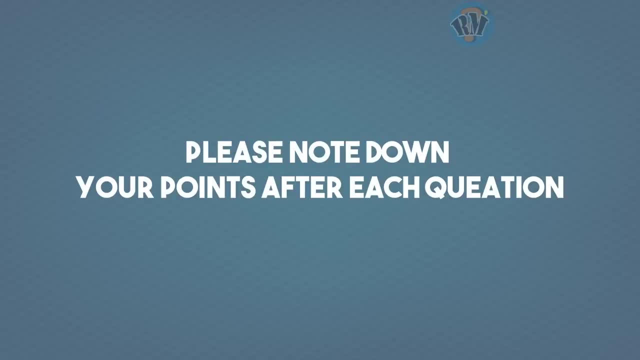 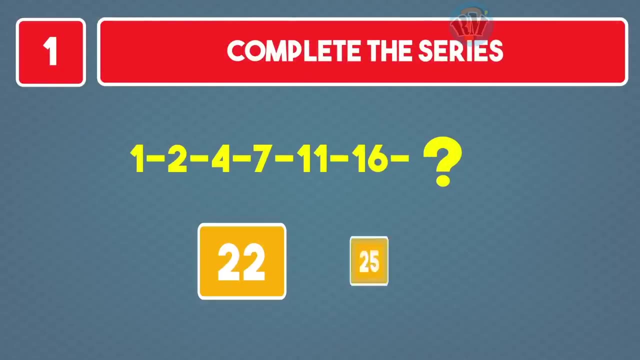 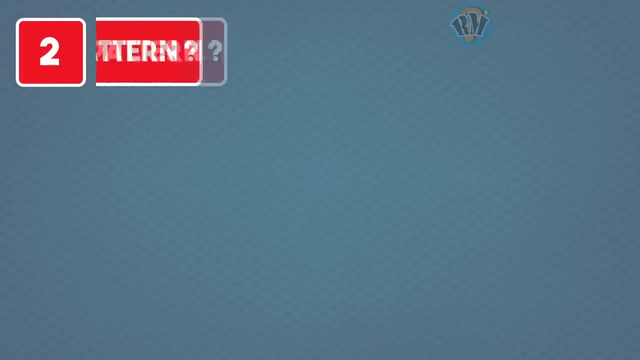 answer and 0 point for incorrect answer. Please note down your score after each question. Let's start the test, Video 2.. You've got a low IQ, so you have to write the test in 3 places. In these 3 places- here the Barack looks great. 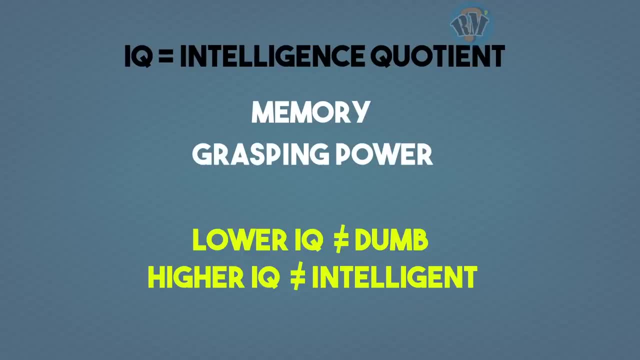 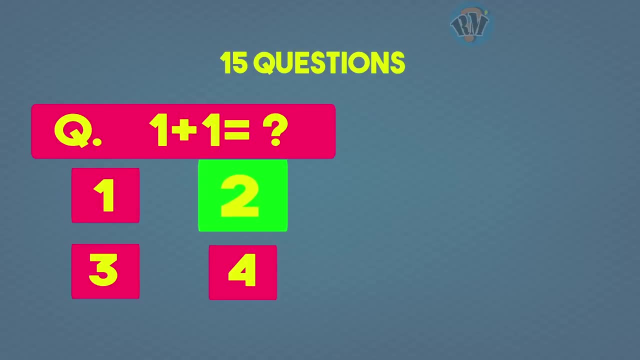 grasping power. Lower IQ does not mean you are dumb. Higher IQ also does not mean you are very intelligent. This test has 15 different types of questions and you have to choose your answers from the provided options. You have 10 seconds to solve each. You will get 1 point for each correct. 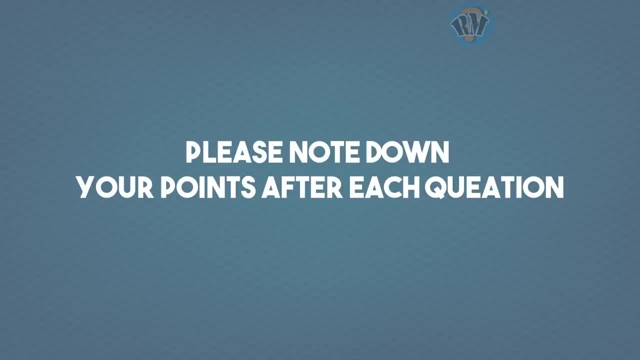 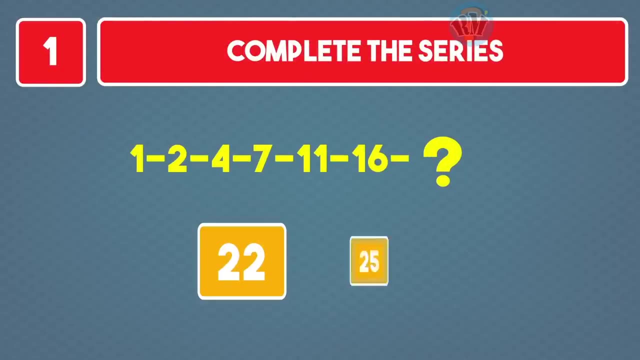 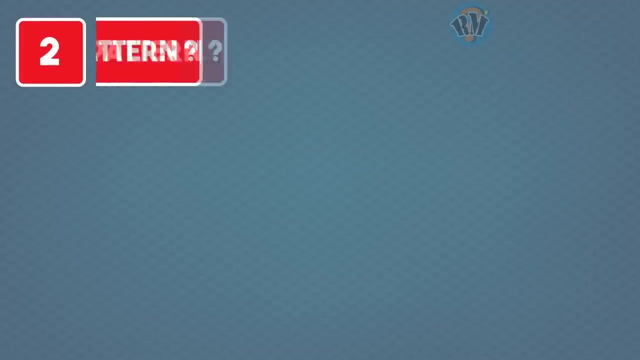 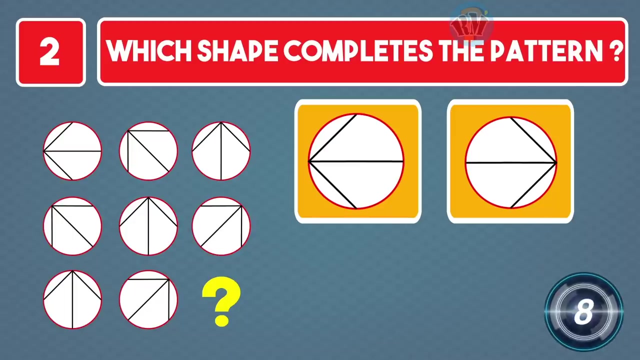 answer and 0 point for incorrect answer. Please note down your score after each question. Let's start the test, Video 2. IQ shows that your IQ is poor, So let's find that out. As soon as the difference in IQ reaches 0, then you pro Entscheidung and you get 0.. 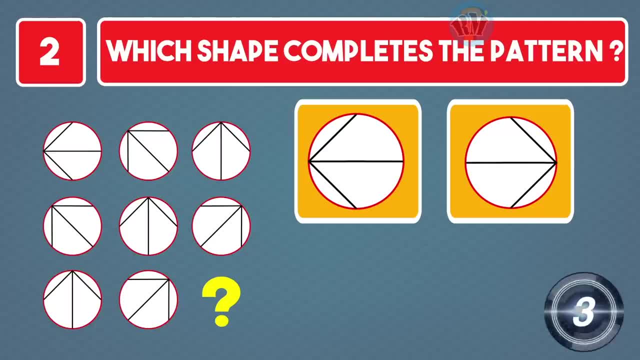 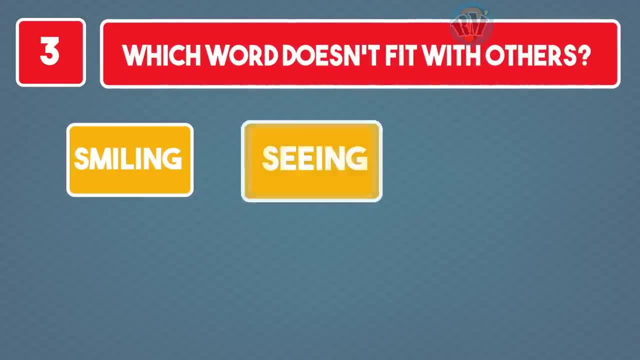 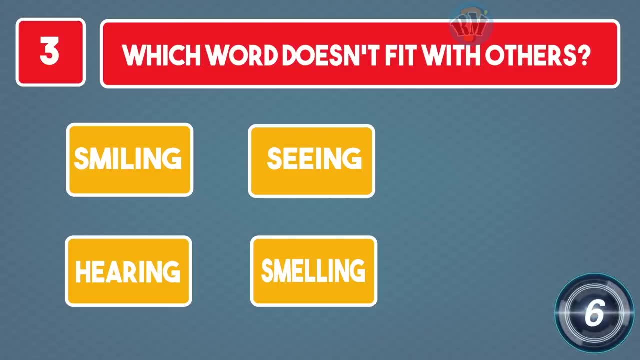 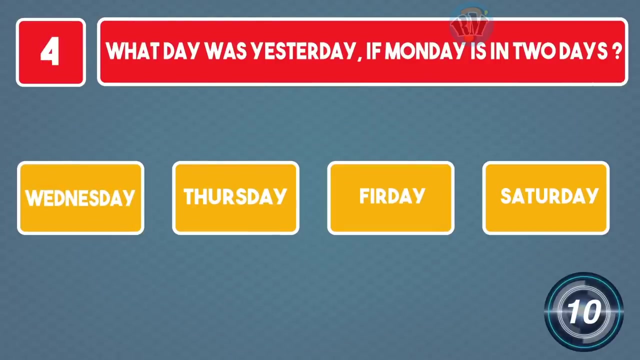 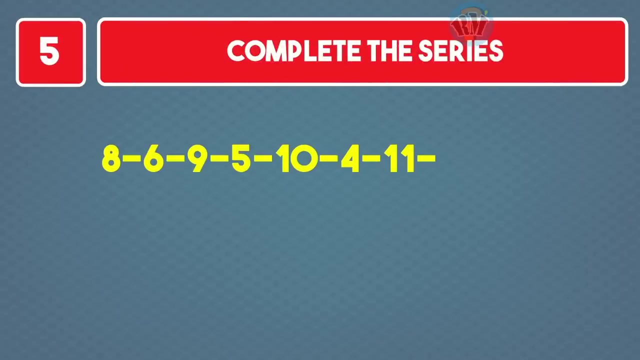 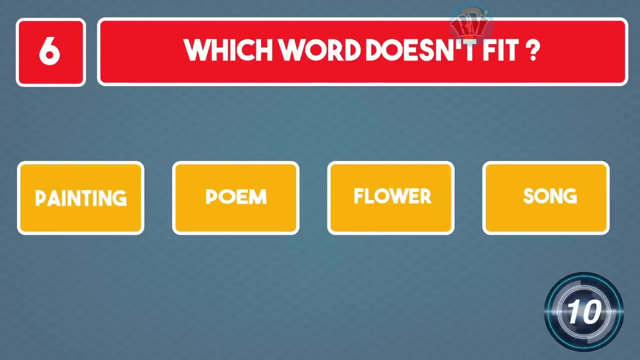 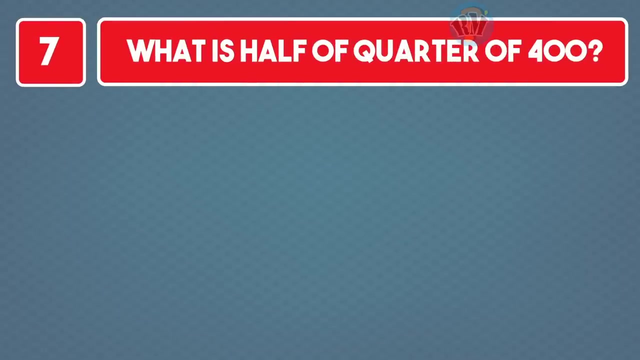 Because it's all in the quiz. you save your time and enjoy the experience of your path. Video 3.. When you have enough IQ to your level, you can study more. You do a good job. Thank you, Thank you, Thank you. 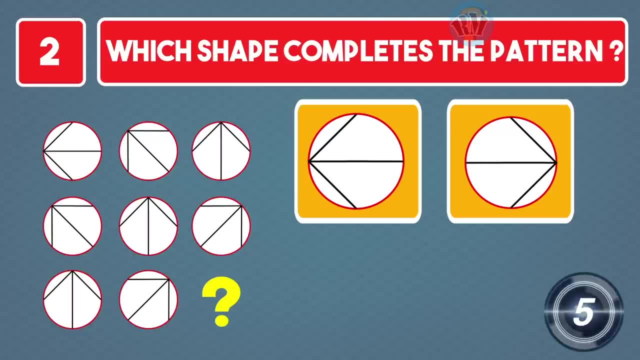 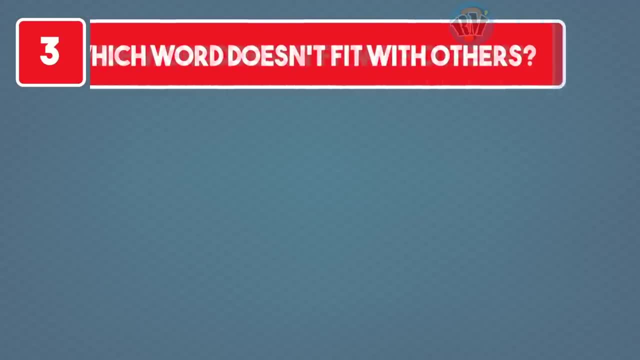 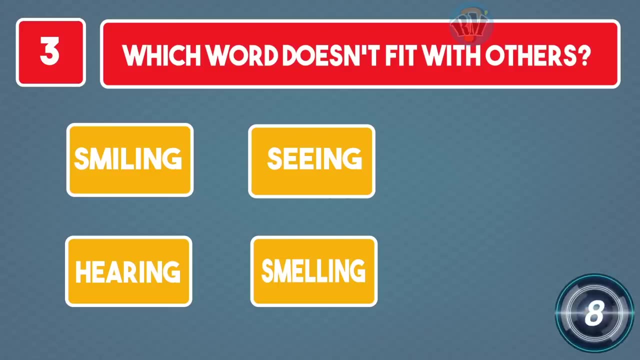 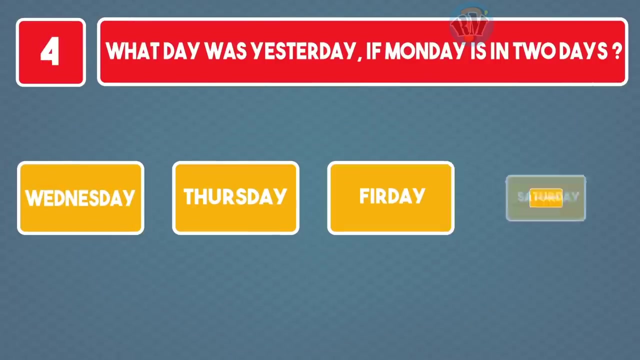 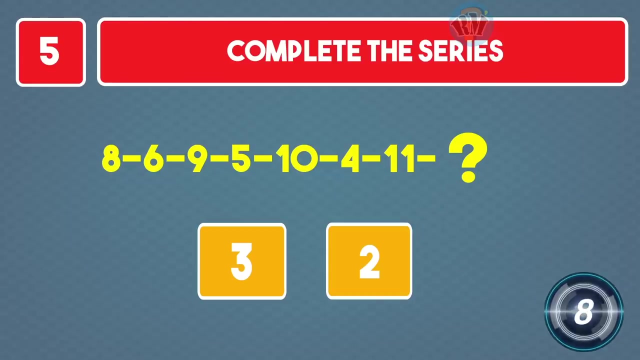 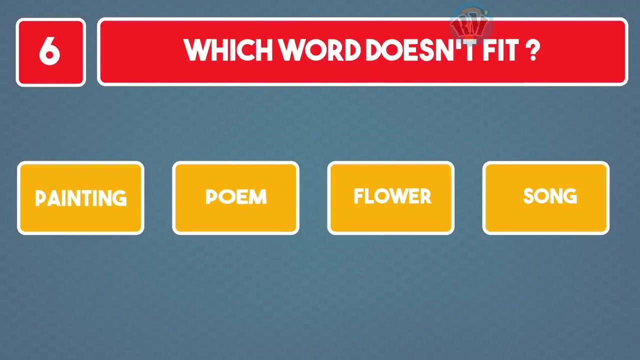 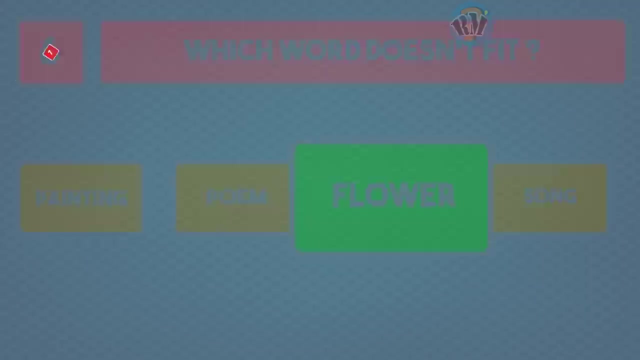 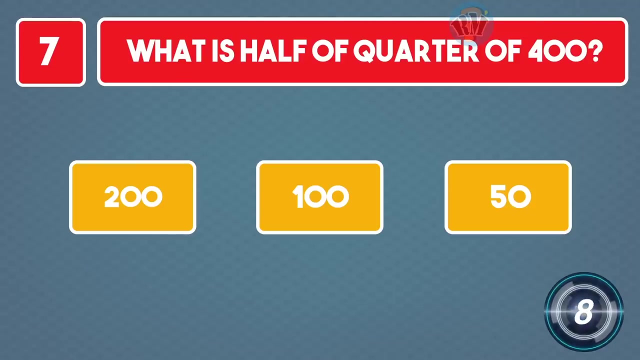 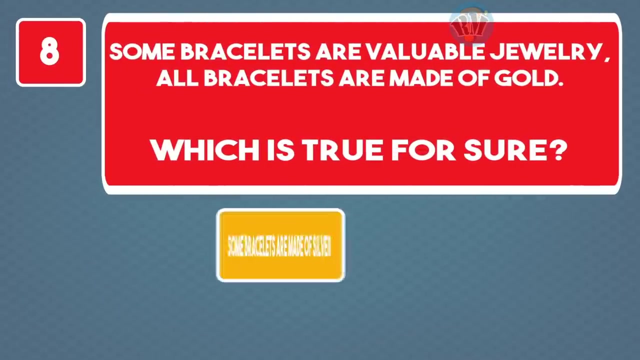 In this level. there is always an IQ aspect to the IQ test Video. 2. There are 5 kinds of Hanes: 1. It Arranges. 2. The Arranges. Thank you, Thank you, Thank you.